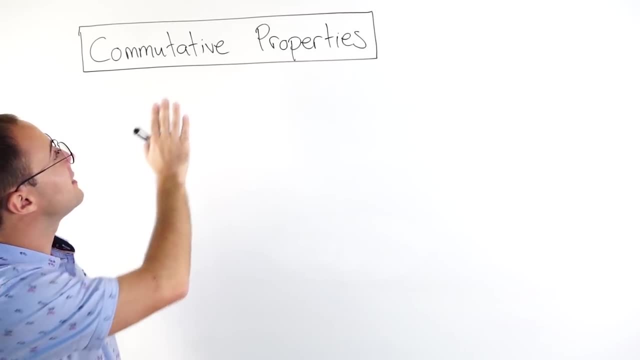 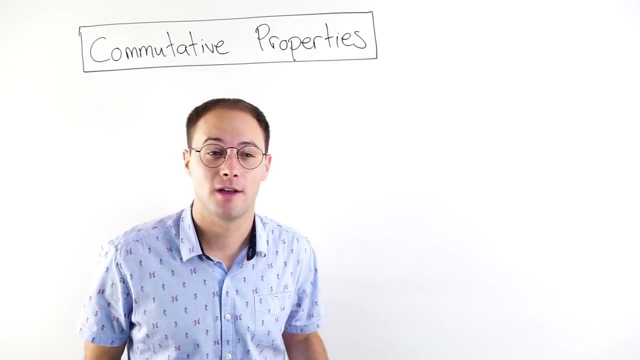 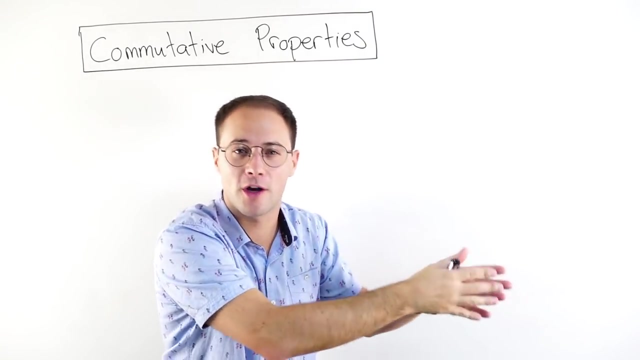 민. Royal character, neau. commutative property. Now, when you look at that word, you might think commute, And if you ask your parents about the word commute, they would probably think about commuting to work. So they would go from their house to work And then when they're done with work, they go from work back to their 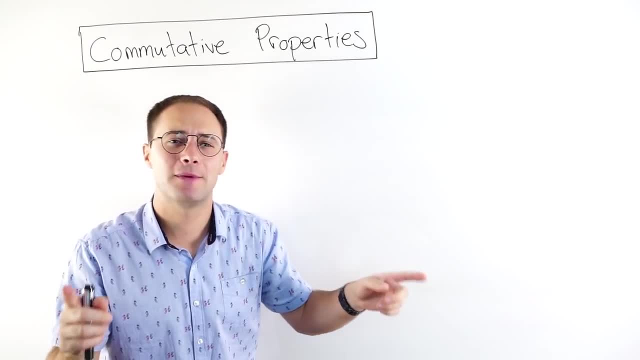 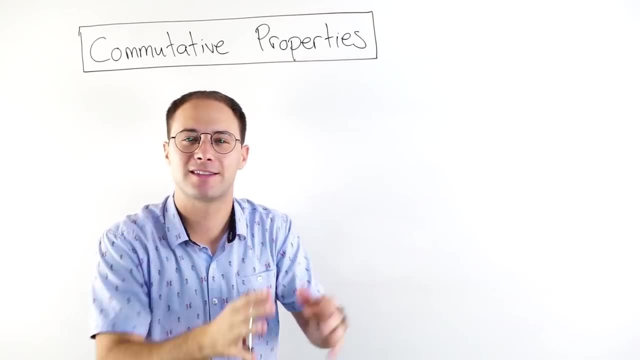 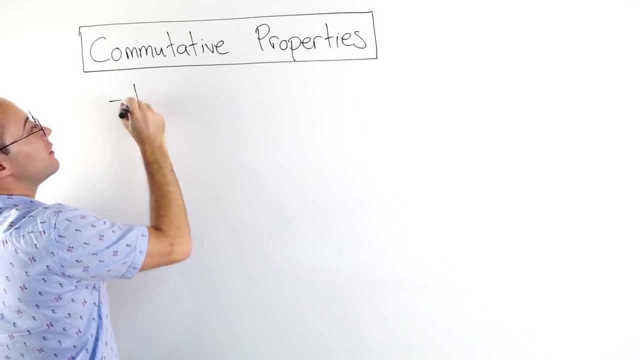 house. Now the distance would always be the same. It's not going to change whether I go from the house to work or work from the house. I could change the order, but the distance is still going to be the same. That's the same thing with the commutative property. The order does not put that. 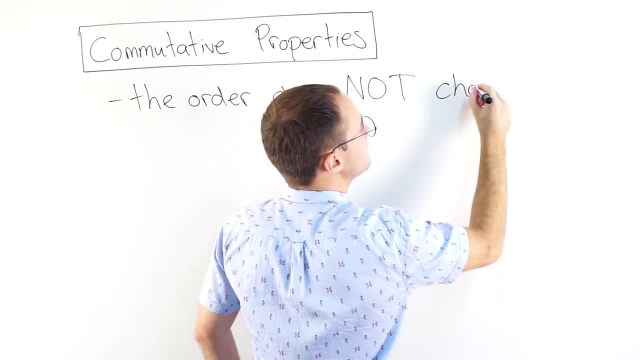 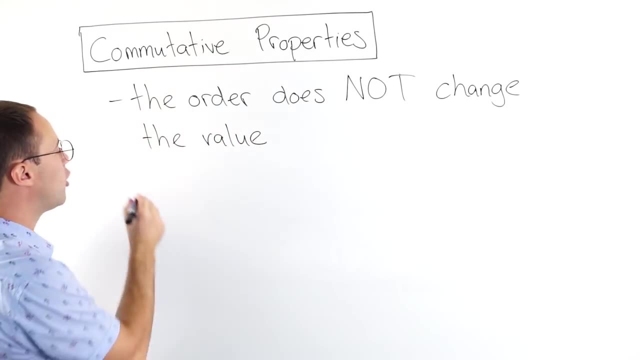 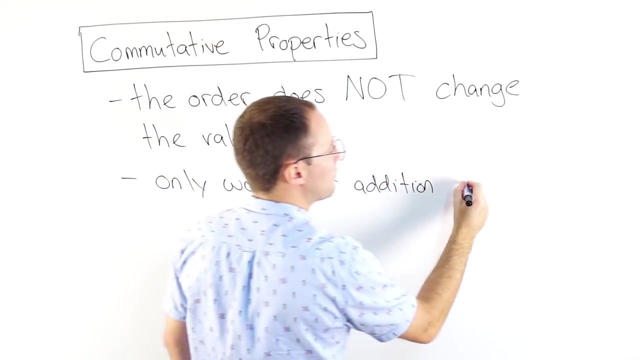 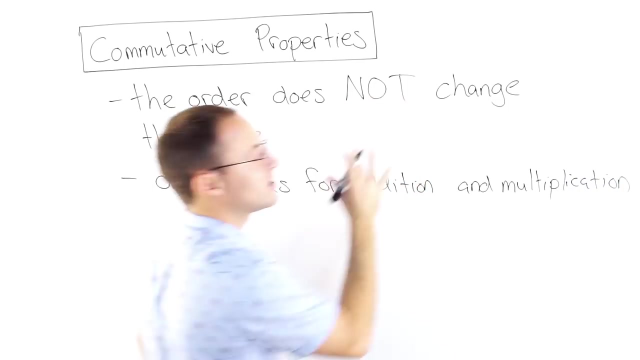 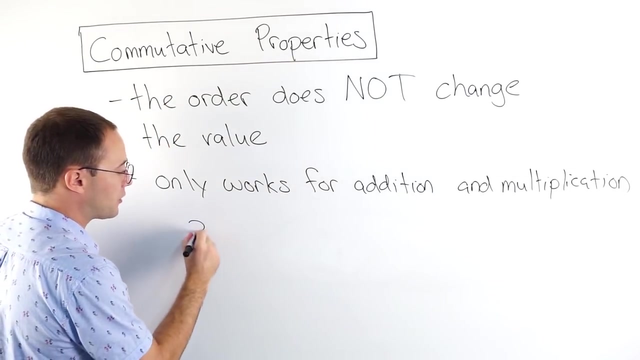 big capital letters does not change the value. The other thing is that it only works with two types of operation, or addition And multiplication. Okay, so make sure you have that written down. So for the commutative property of addition, we could have something like three plus two. Well, that expression is equivalent. 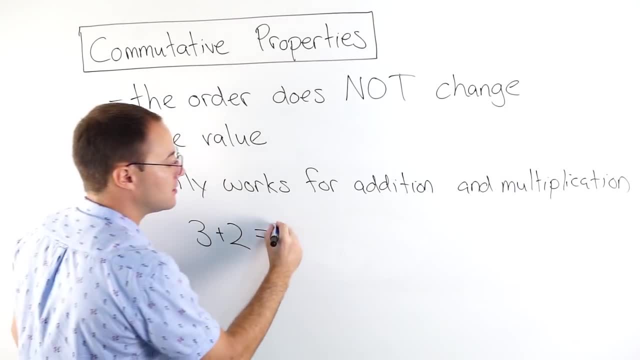 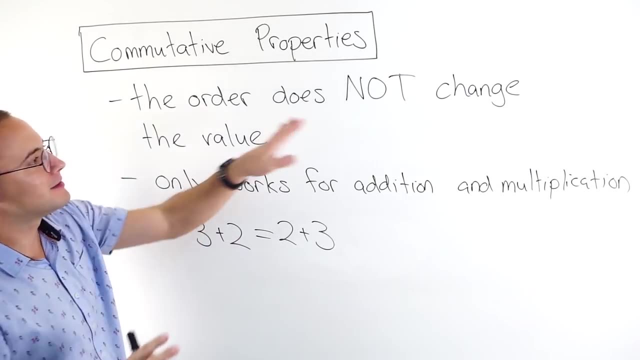 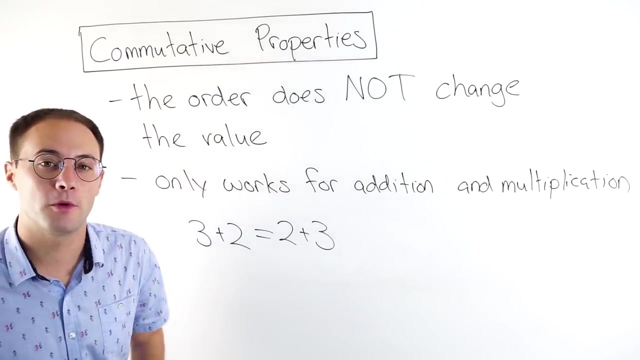 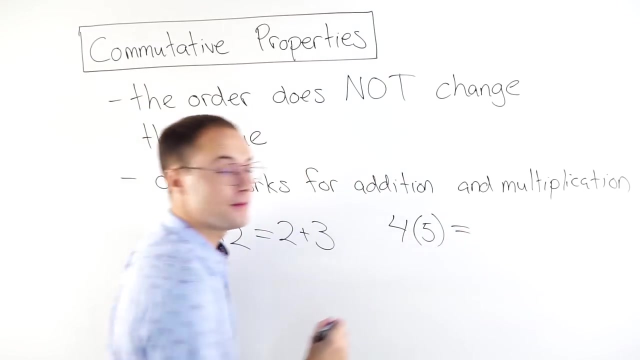 right, It has the same value as two plus three. Okay, we change the order. the value does not change. Three plus two is five. two plus three is five. The value is still the same. It works for addition. It can also work for multiplication. Four times five is equivalent to five times. 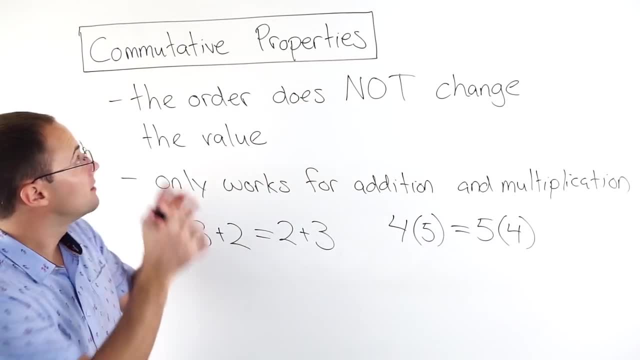 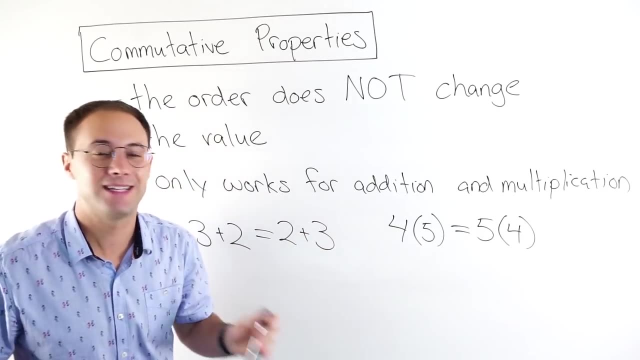 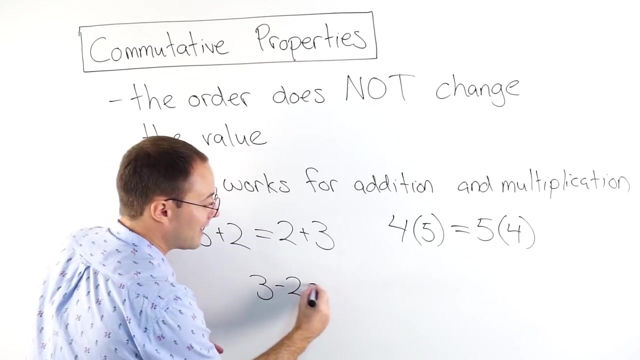 four. They both have the same value For commutative property. the order does not change the value. Order does not matter And it only works for addition and multiplication. Right, If I try to do subtraction, three minus two is not equal to two minus three. three minus two is one. 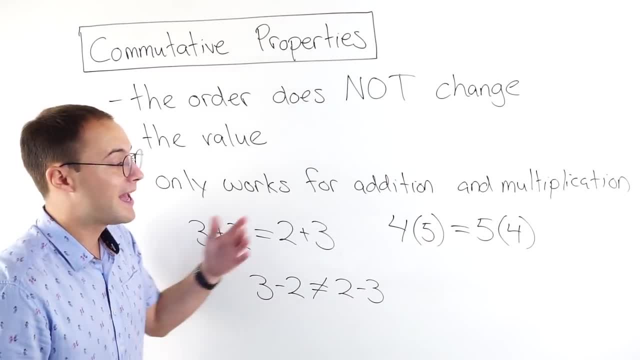 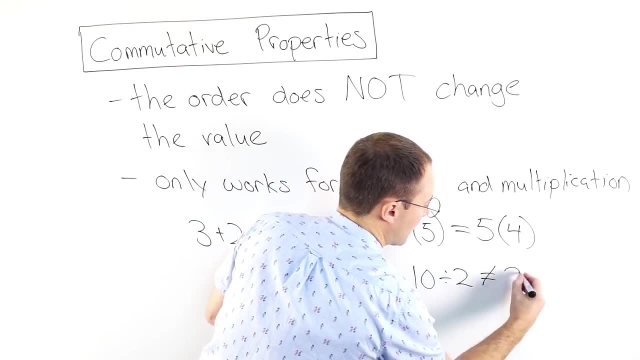 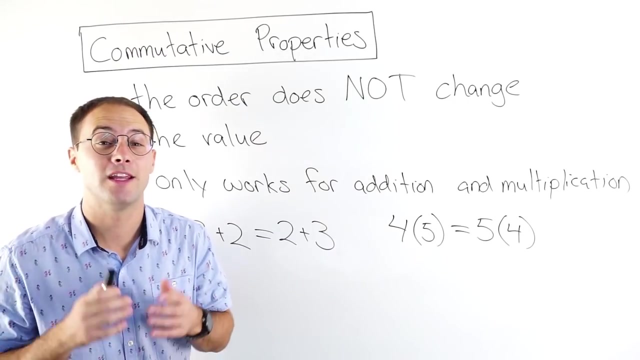 two minus three is negative one, So that doesn't work. And same thing with division: 10 divided by two is not the same as two divided by 10.. They don't have the same value. They are not equivalent. Let's check out the associative property. All right, let's go back to the commutative property. Okay, let's go back to the commutative property. Okay, let's go back to the commutative property. All right, let's go back to the commutative property. 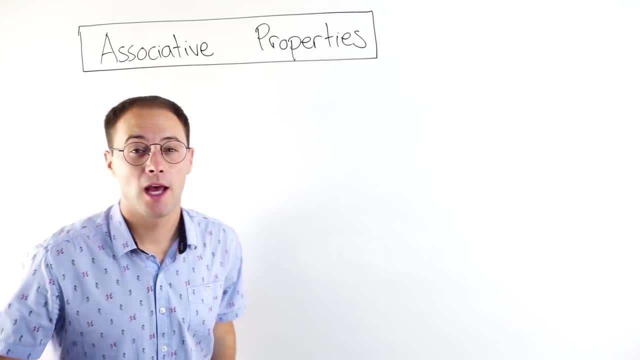 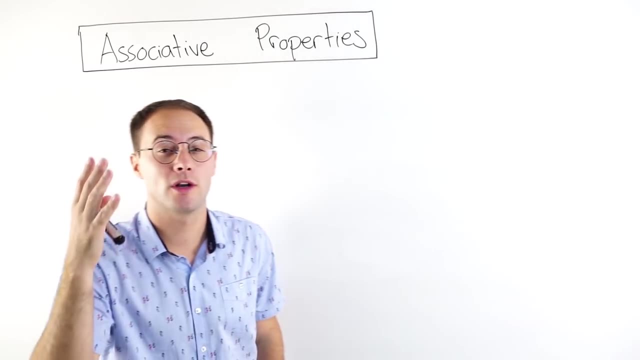 All right, let's talk about the second property, the associative property. Well, just like we did with commutative property, we talked about the word commute, Associative property let's talk about the word associate. Associate just means: what do you identify with If I want to give myself as an? 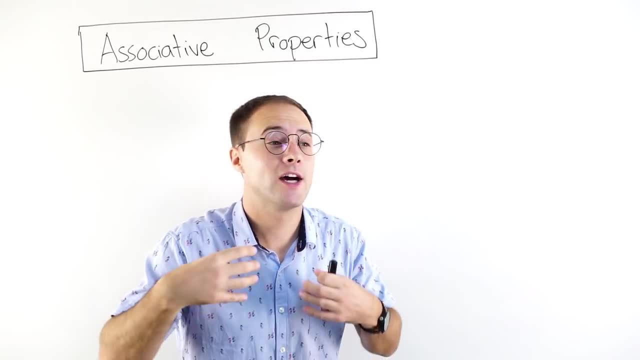 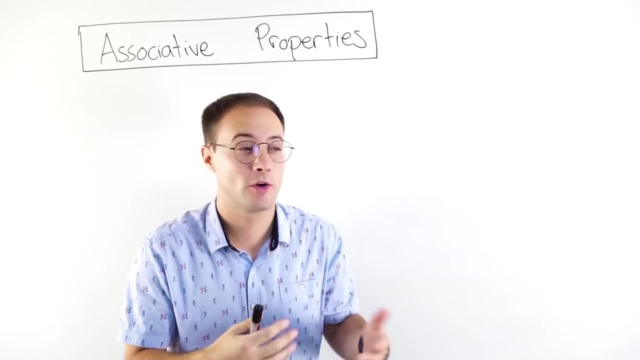 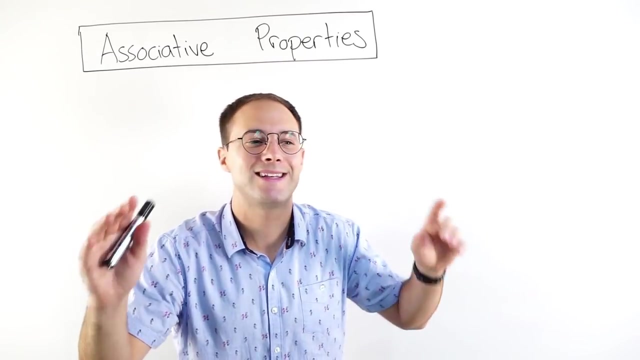 example, I like to play soccer, So I associate myself with soccer players or with my team. I also like to snowboard in the winter, So in the winter I might associate myself with other snowboarders, Depending on what group I'm in. it doesn't change who I am, I'm still. 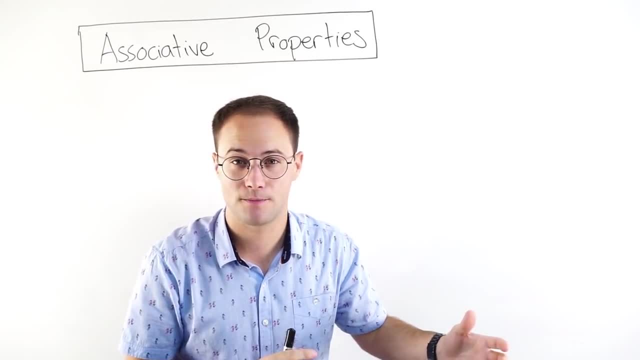 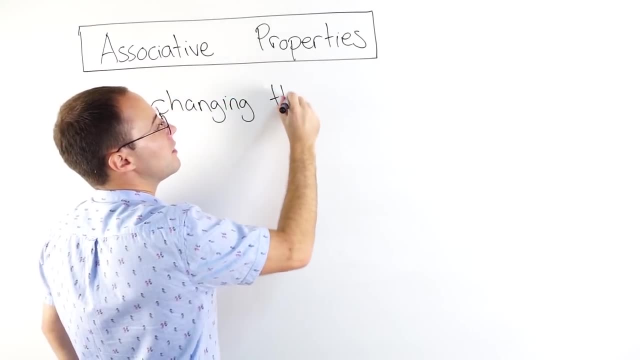 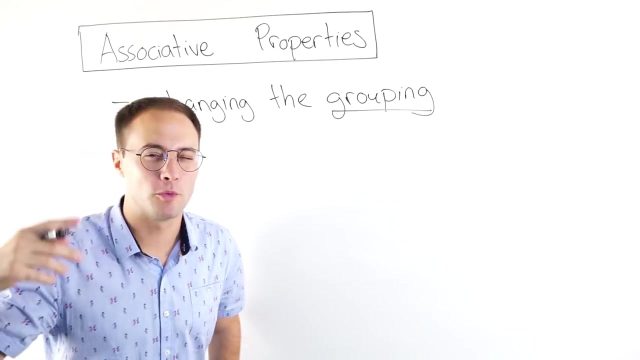 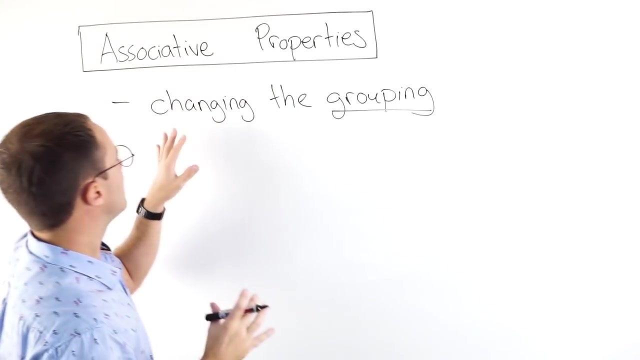 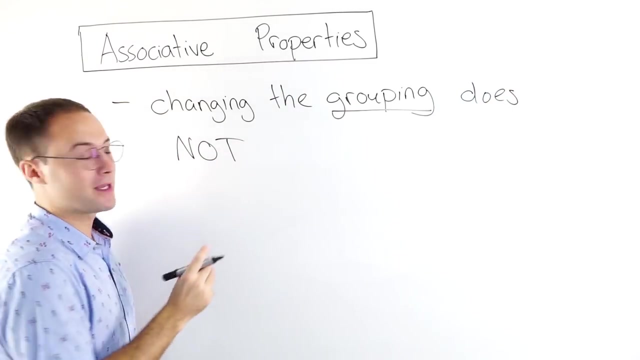 myself. I haven't changed, but the grouping has changed. So the associative property is changing the grouping. So whenever you think of associative property, think of groups. right, Do I kind of associate myself with the soccer group or the snowboarding group? right, Changing the grouping does not. again big capital letters. 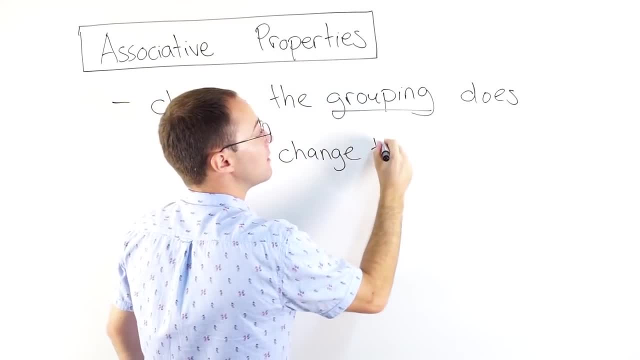 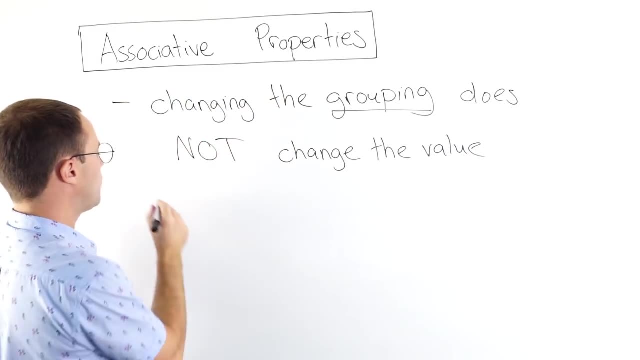 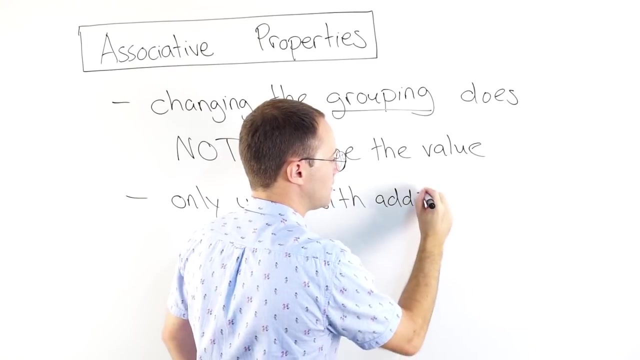 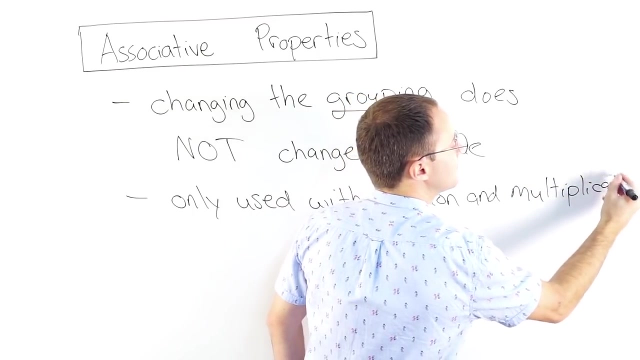 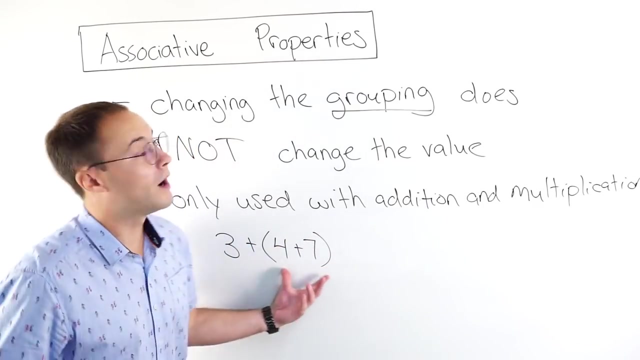 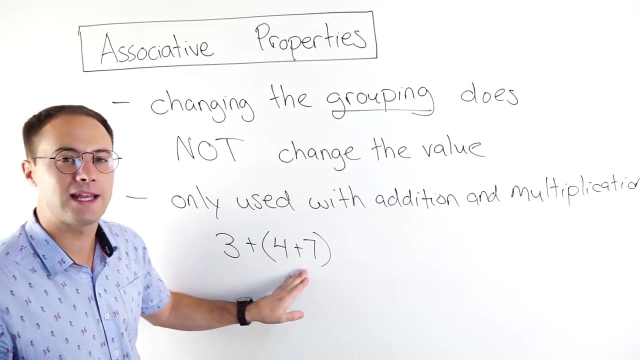 does not change the value. okay, And this is just like the commutative property. We only use this with addition, Addition, Multiplication. If I had three plus four plus seven, well, right now we're grouping four plus seven together, But because this is all addition, we're only adding here. that would be equivalent. 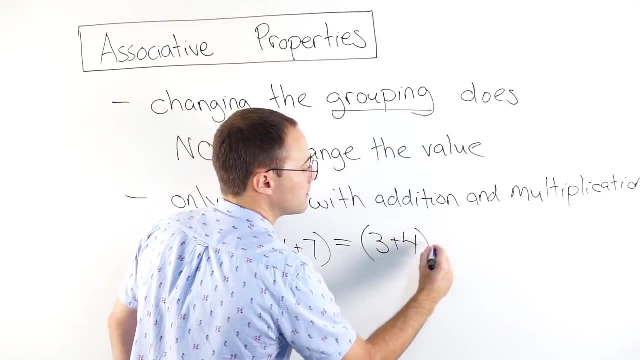 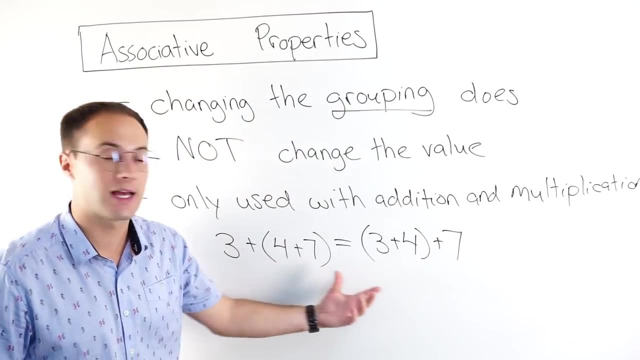 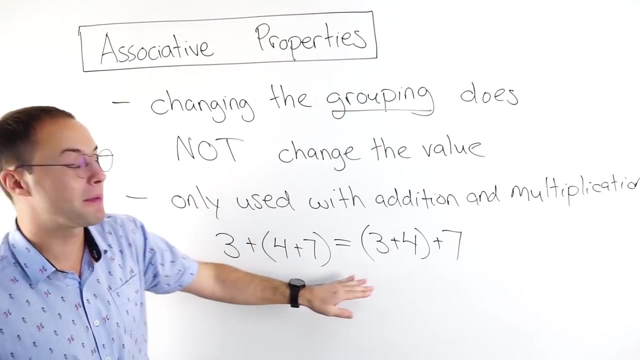 to three plus four plus seven. I could decide to group the three plus the four together instead of the four plus the seven. Those are equivalent expressions Right here we just demonstrated the associative property of addition, Same thing with multiplication Three times ten. 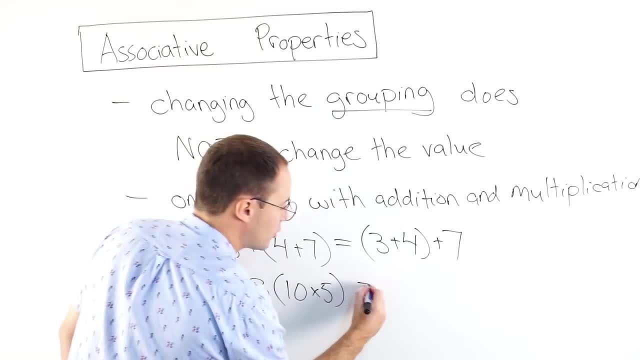 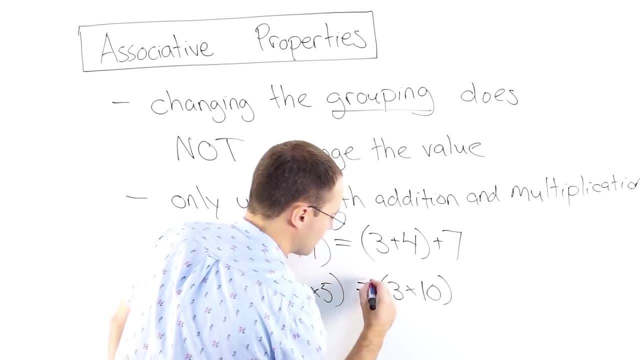 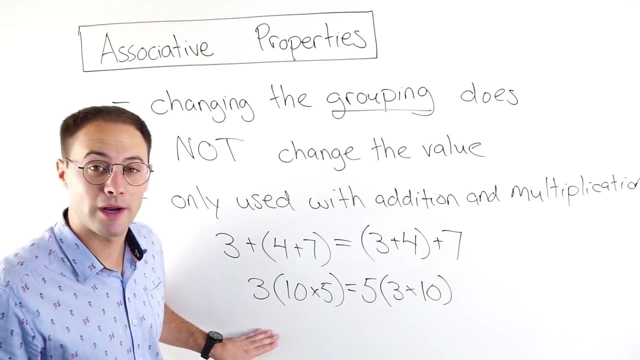 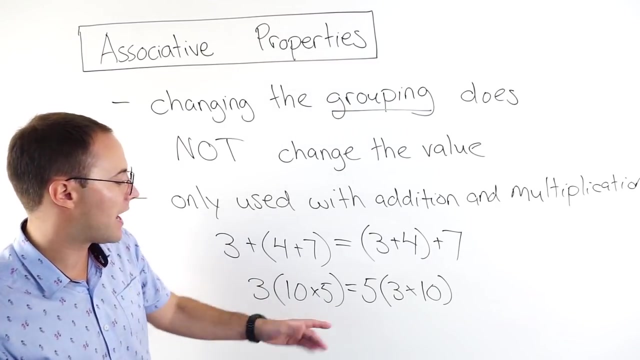 times five, That's equivalent to three times ten times five, And I'll put the five out front. Those are equivalent expressions as well, because this is all being multiplied together. So changing the grouping is not going to change the value. Ten times five is fifty times five, sorry times three. 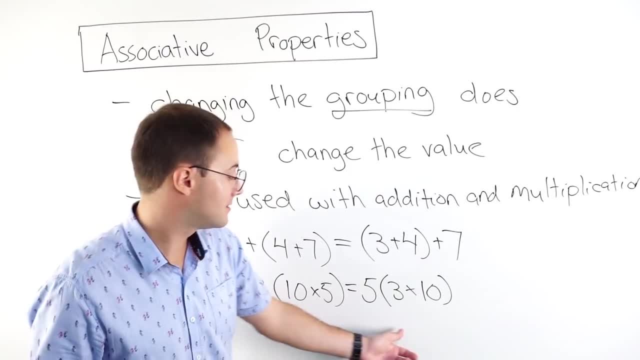 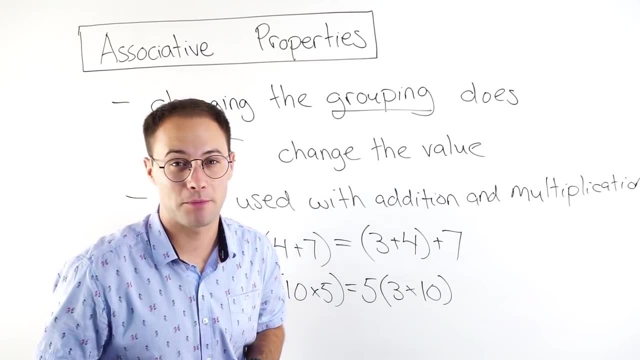 is a hundred and fifty. Three times ten is thirty times five is a hundred and fifty. The value is the same. They are equivalent expressions. Let's get into some examples. Alright, here we go with example one. Simplify the expression and explain each step. 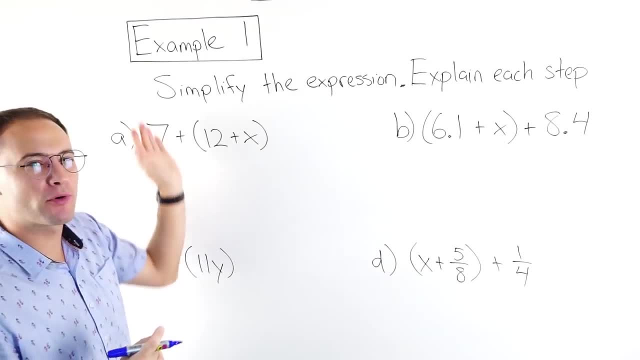 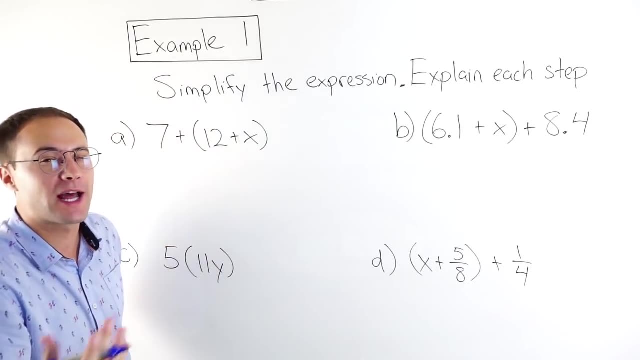 So A we've got seven plus- in parentheses- twelve plus x. Well, I can't add twelve plus x because x is a variable. I don't know what it actually is, I don't know the value of it, But I could do. 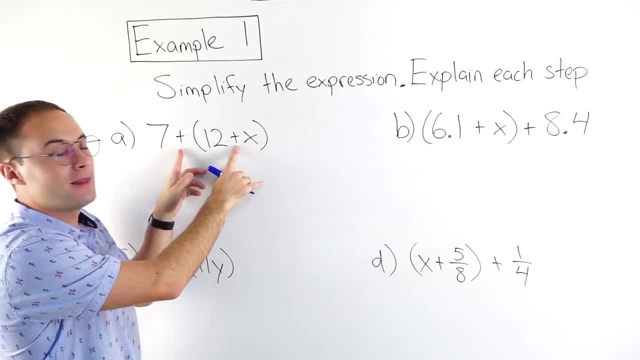 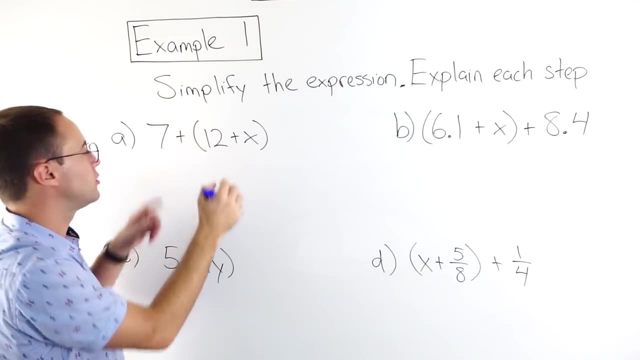 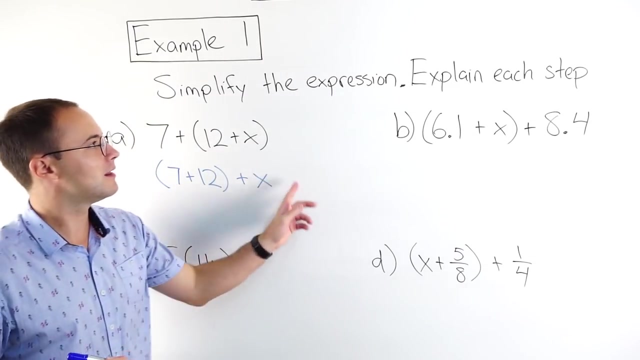 seven plus twelve, And, if I notice, we're only using addition. So in that case, instead of having these grouped together, I could change the grouping to this: Seven plus twelve and then plus x. Well, we're simplifying. Let's explain this step. What step did we just use? 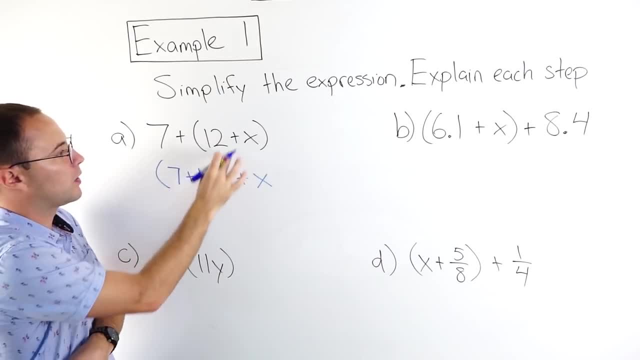 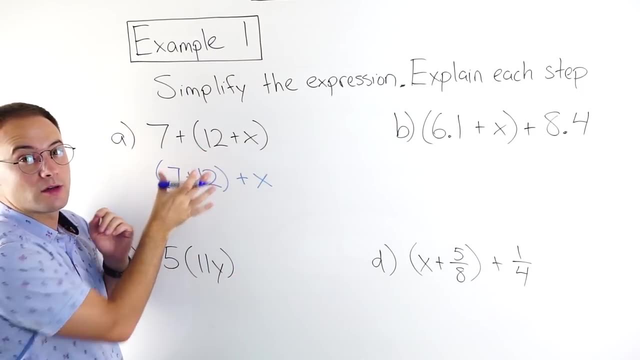 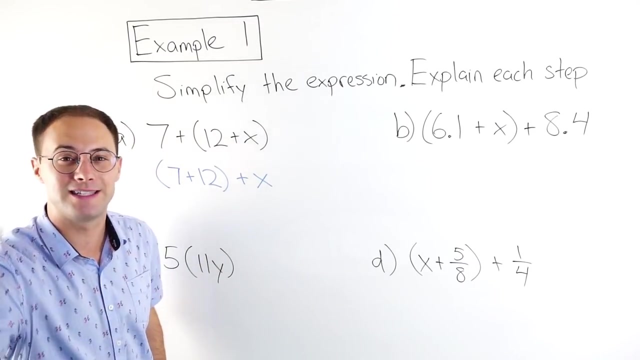 We changed. we didn't change any of the order. seven twelve x. The order didn't change, so it's not commutative property. The grouping changed right, So that's associative property And if you think this is addition, so it's associative property of addition. I'm just going to write A P, A. 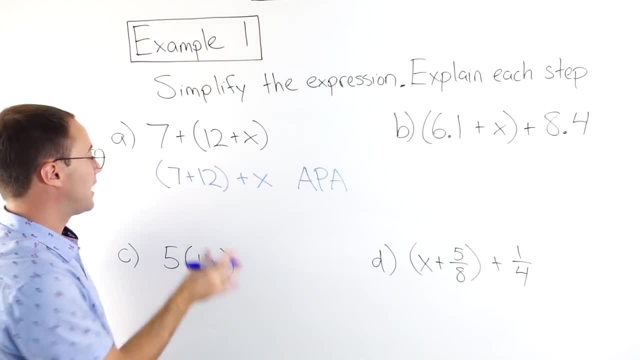 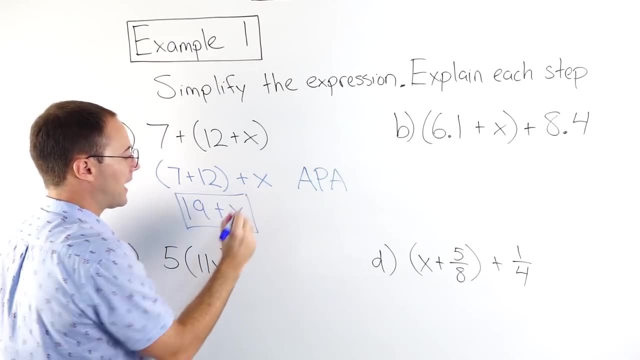 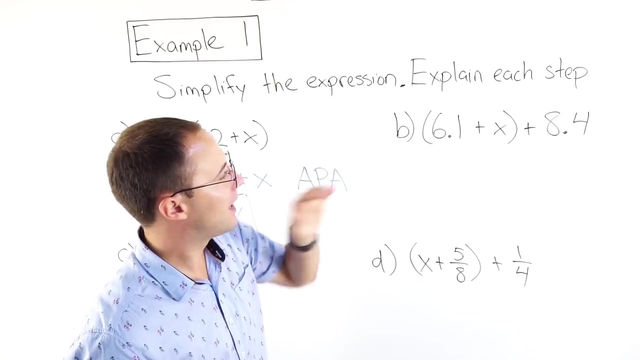 It's not commutative property of addition. Okay, Now let's simplify. Well, seven plus twelve is nineteen plus x. So now that is simplified, Let's go to the next one: Six point one plus x, plus eight point four, It's all addition. so I know I'm going to be using one of the properties of 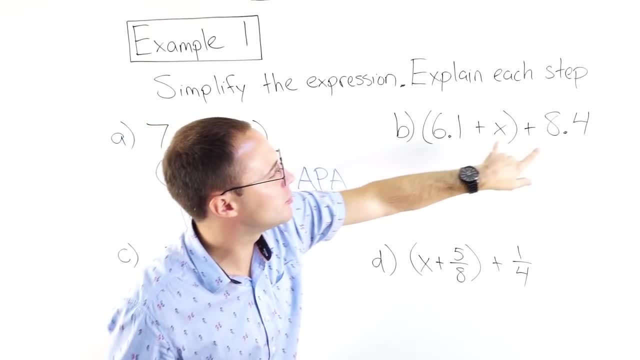 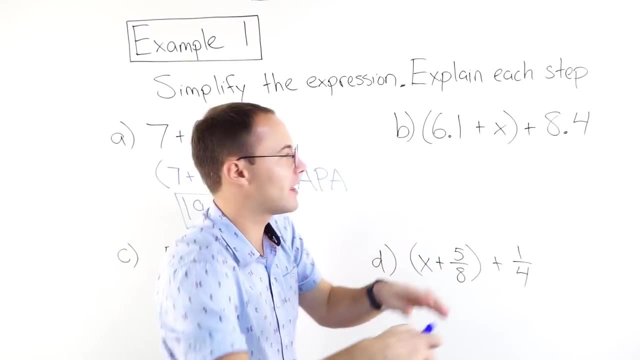 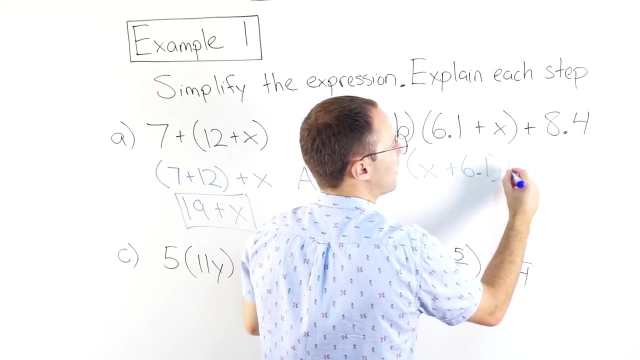 addition. But I want to do eight point four plus six point one. Well, first I should change the order so I can group them together after that. So let's change the order. So let's make this x plus six point one and then plus eight point four. So all I did was change the order. So we know that. 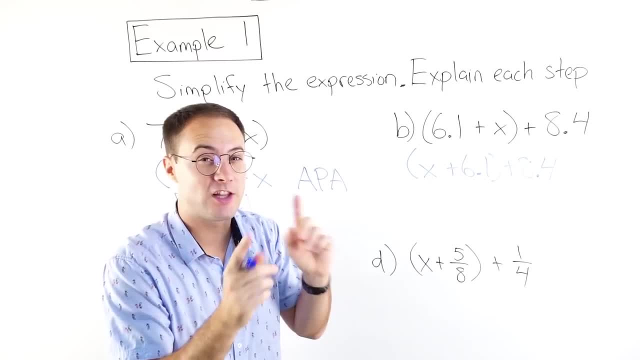 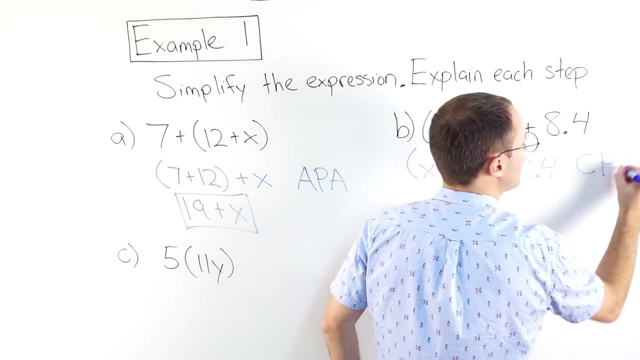 that one was commutative property. Commutative property was changing the order and you keep the same value. So commutative property of addition- I'm just going to say commutative property, addition. CPA, like a certified public accountant. 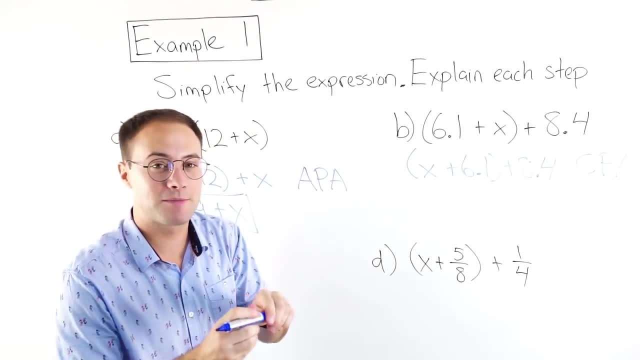 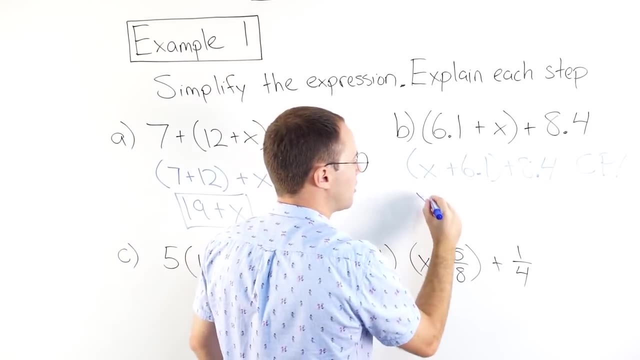 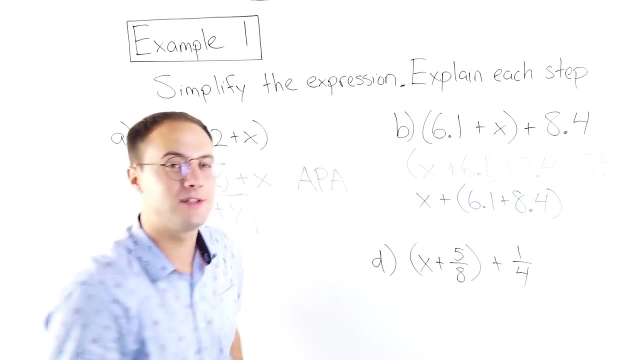 Now we still have another step to do. We still haven't simplified yet. Again, like I said before, I want to group these together. So let's change the grouping. Let's go x plus six, point one plus eight point four. We're grouping those two decimals together. Change the grouping, That's. 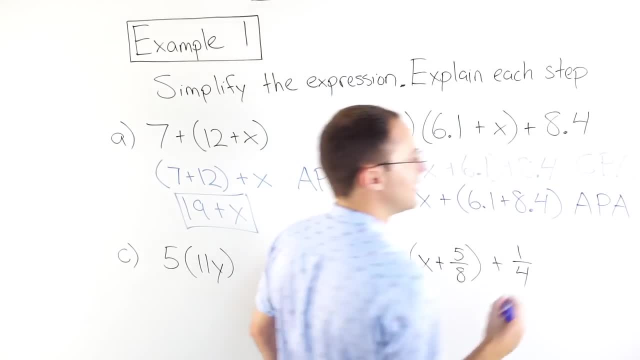 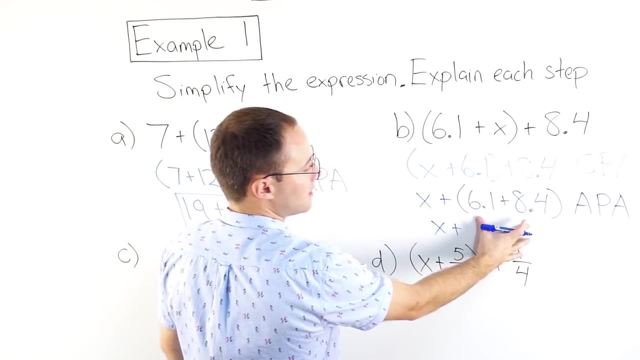 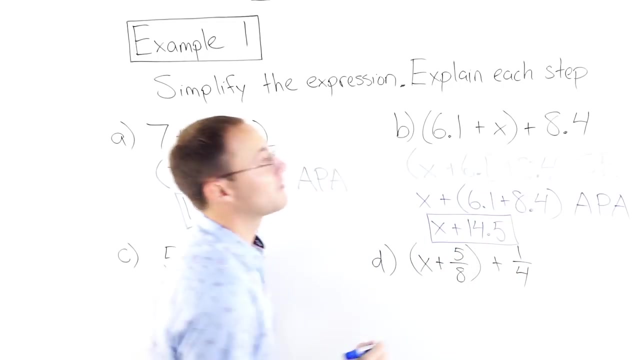 associative property. of addition, Remember explaining your steps as you go. And now we can just add those together. So I get x plus… plus, what is that? 14.5?, 14.5.. There's my simplified expression. 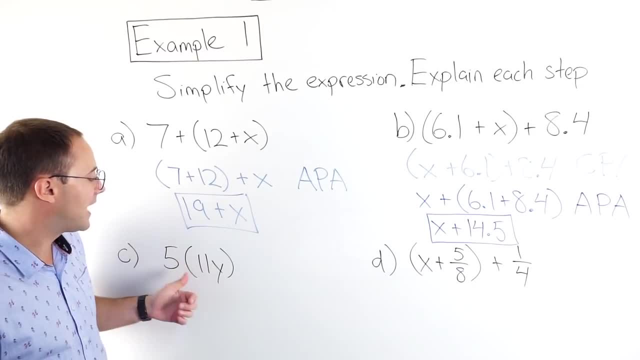 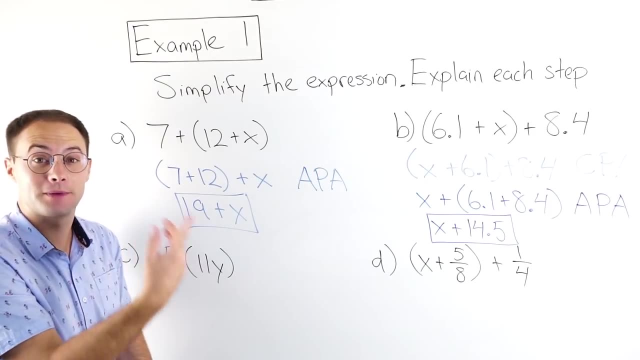 Okay, Let's go to the next one: C, 5 times in parentheses, 11y. Now remember: if you have a number next to a parentheses, that means multiplication. If you have a number next to a variable, that also means multiplication. 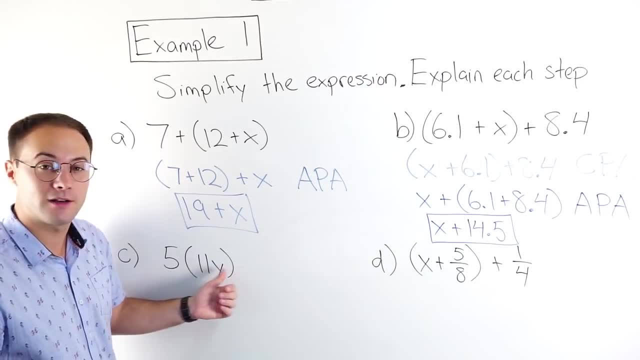 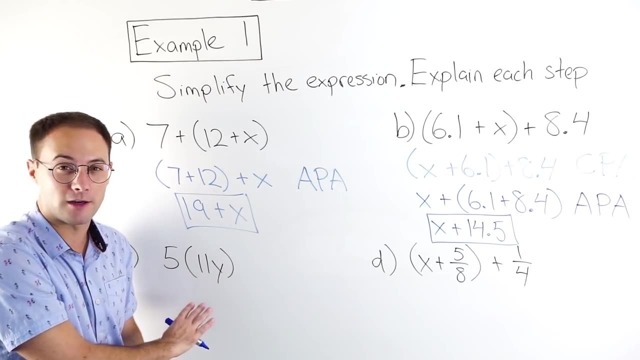 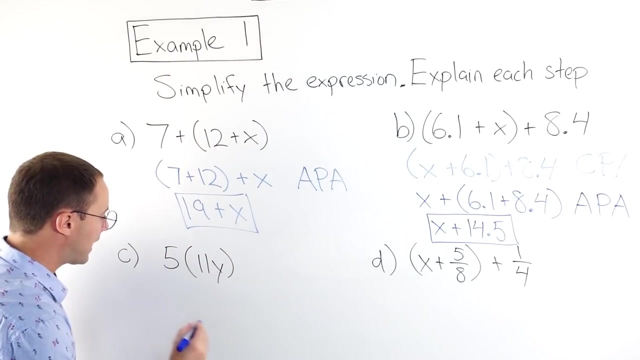 And we call that a coefficient. Remember, coefficient that means we're multiplying it by that variable Multiplication, multiplication we're only multiplying here. So that allows us to do either the commutative property or associative property, or both. So I'm going to have 5 times 11 and then times y. 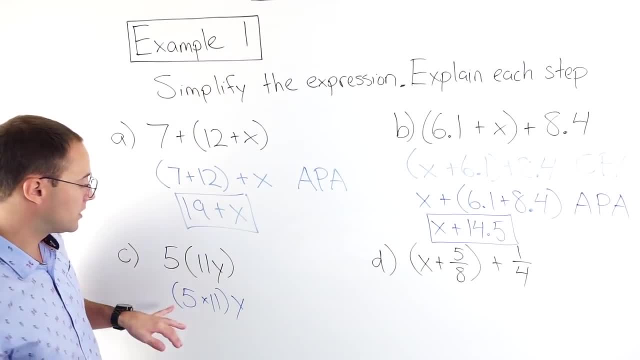 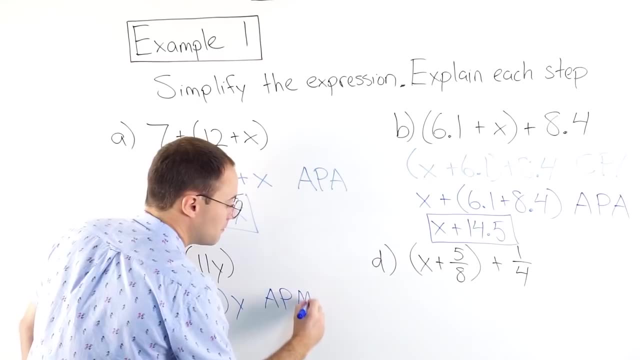 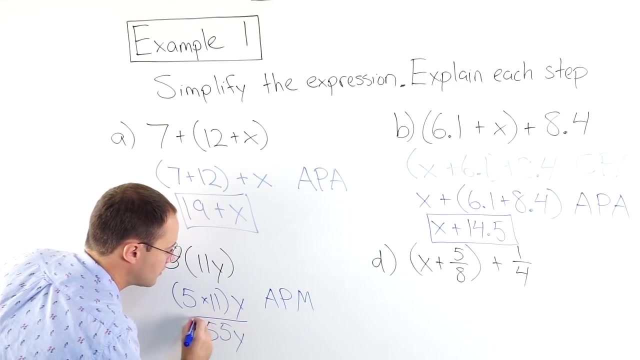 Okay, Because I can do 5 times 11.. So all I did was change the grouping That's associative property of this time multiplication Now 5 times 11, that's simple, 55 times y, so 55y. 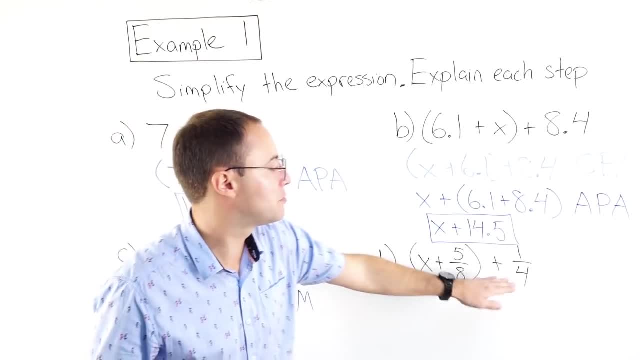 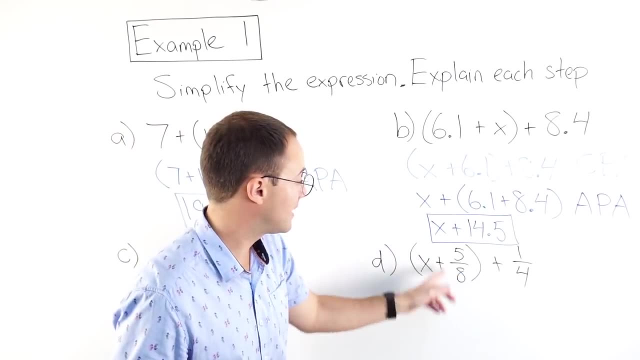 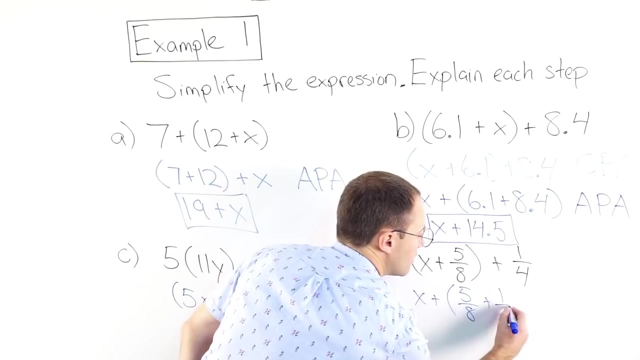 Last one: x plus 5 eighths in parentheses, plus 1 fourth at the end. Again, I want to change the grouping Here. the order's fine, I can keep that order and just change the grouping. So I'll go x plus, in parentheses, 5 eighths plus 1 fourth. 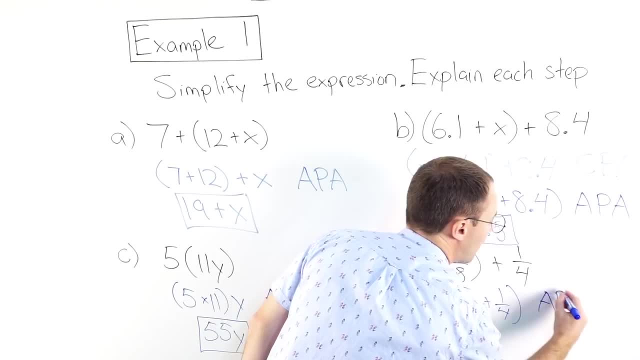 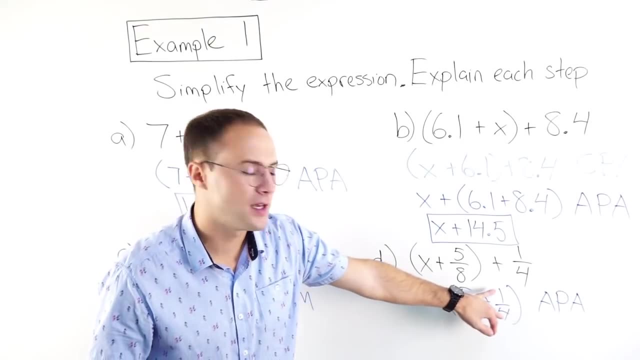 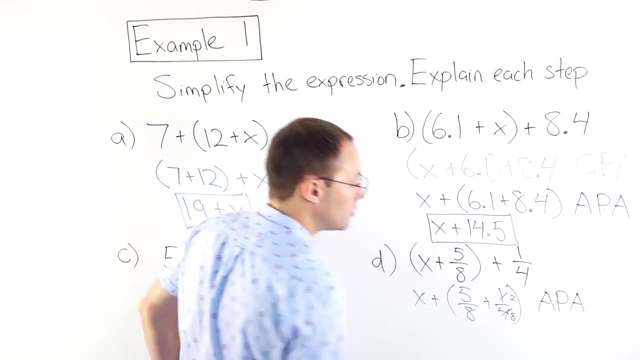 I just changed the grouping, That's associative property of addition. Okay, And now let's add: Well, 5 eighths plus 1 fourth. I need a common denominator. So that's going to become 8, and that's going to become a 2..